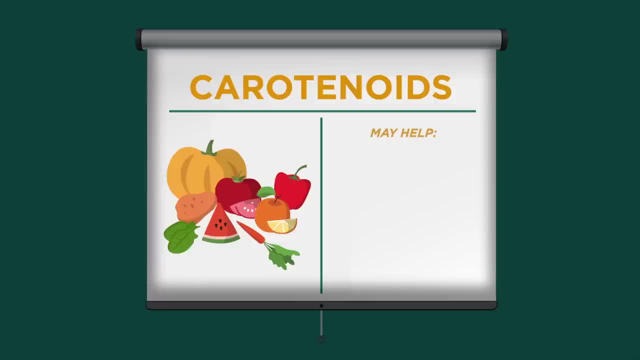 These colorful plant pigments found in bright red, yellow and orange fruits and vegetables act as powerful antioxidants and may help prevent some types of cancer and heart disease, reduce the risk of eye disease, enhance the immune system and more. Resveratrol is another bioactive found in the skin of grapes, blueberries, raspberries and mulberries that may reduce the risk of heart disease. 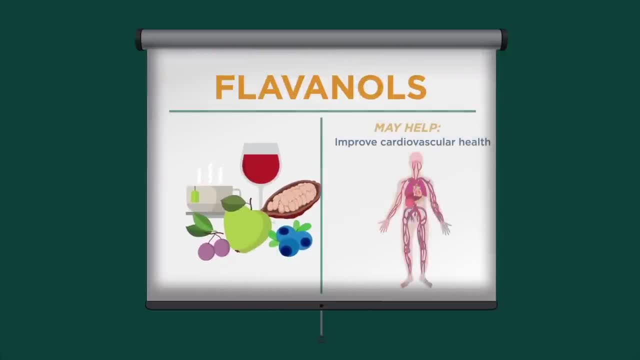 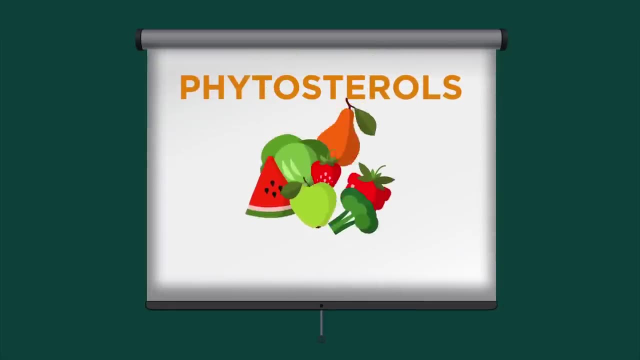 Flavanols are a part of the flavonoid family that are found in tea, red wine and cocoa and may positively influence our cardiovascular health. Phytosterols are steroid compounds in plants that may lower cholesterol and improve cardiovascular health. Phytoestrogens found in many plants, including soy and other legumes, are also being studied for their properties. 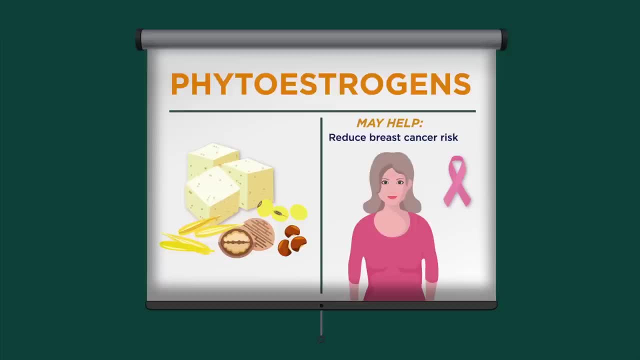 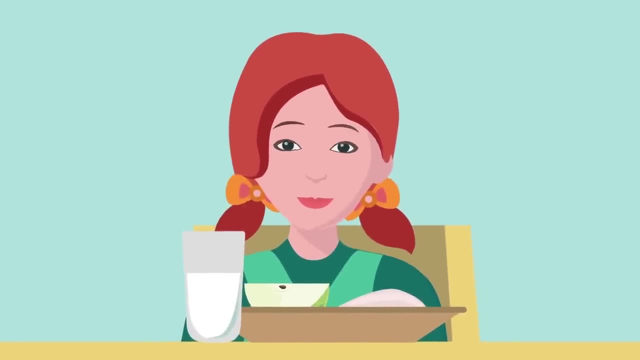 Phytoestrogens are also being studied for their potential in reducing the risk of breast cancer. Healthy eating is important at every age, but the amount of nutrients we need and our body's ability to process them can change over time and depend on your personal health status. 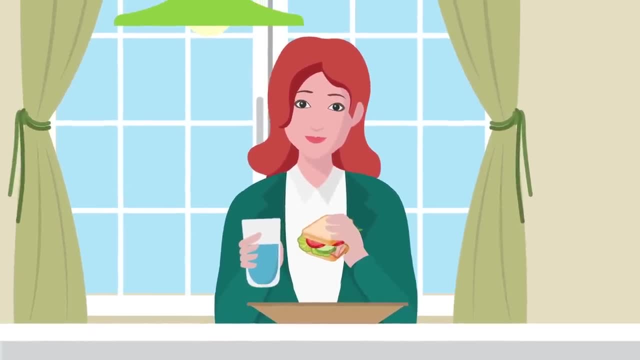 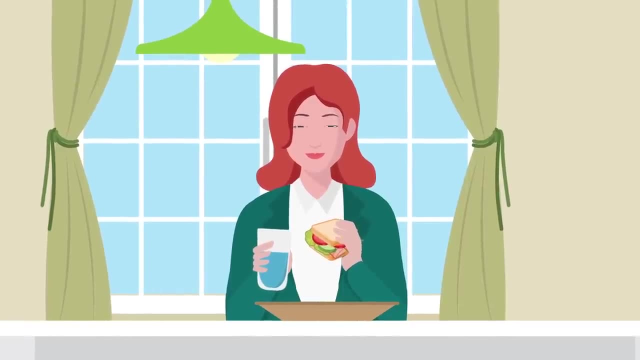 As you age, you may need more vitamin D and calcium for bone health, more B12 for brain and blood health and more fiber for a healthy digestive system. Some people may also need more water as their sense of thirst declines. Your medical conditions or the medications you take are important. 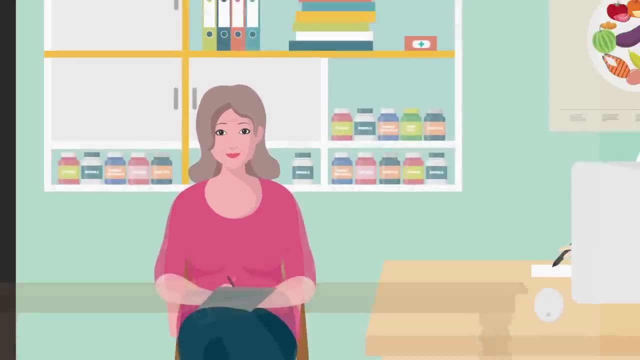 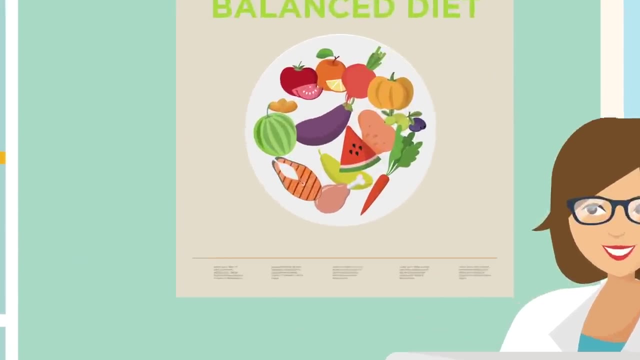 It's important to talk with your health care team when deciding the best nutrition plan for you, But most people can get the healthy nutrients they need from a well-rounded diet of nutrient-rich fruits and vegetables, lean proteins and whole grains such as those recommended in the US Dietary Guidelines. 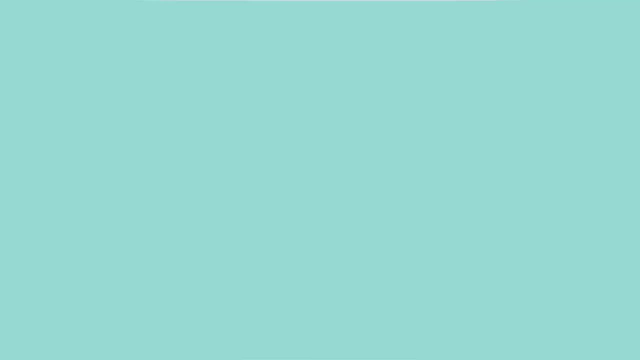 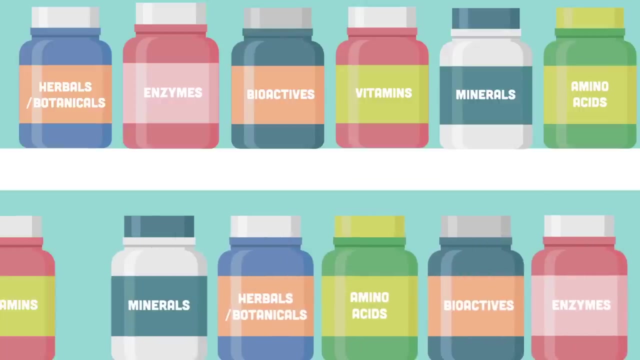 Some people with deficiencies, certain diseases and conditions, or with evolving nutritional needs at different stages of life may consider dietary supplements to add missing nutrition to their diets. Supplements include vitamins, minerals, herbals and botanicals, amino acids, enzymes and bioactives. 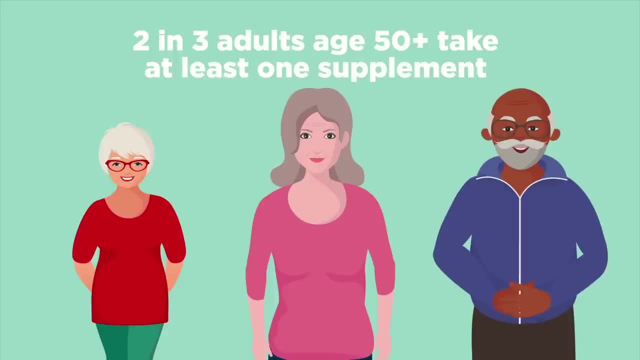 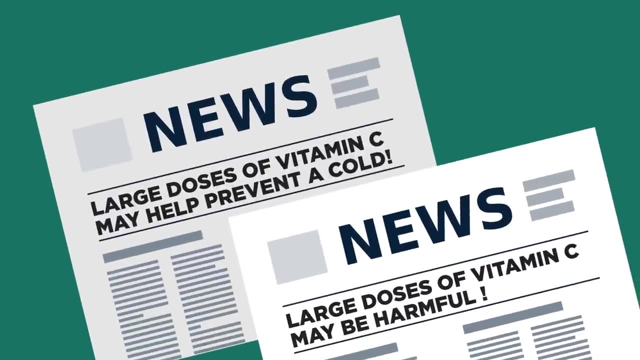 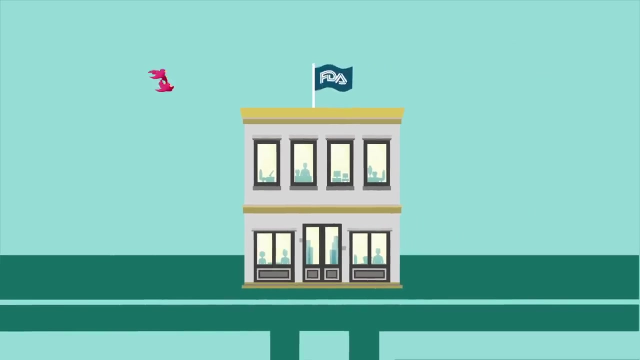 You may be one of the many adults that takes a dietary supplement of some kind, but do you know enough about what is safe and what you can trust? Too often, what's popular one day seems to make headlines the next for being unsafe. The Food and Drug Administration that regulates the safety and effectiveness of our drugs and medical devices also regulates dietary supplements.